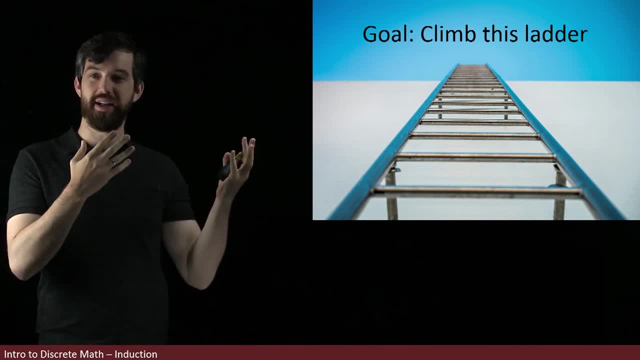 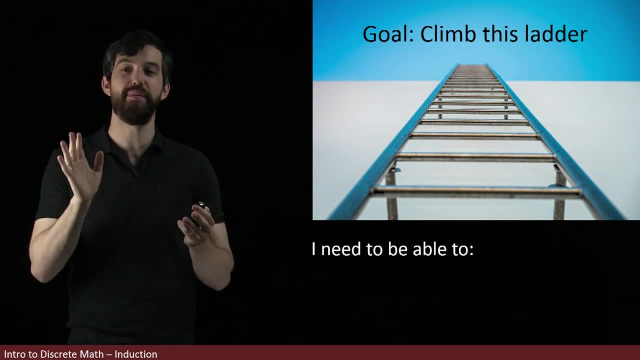 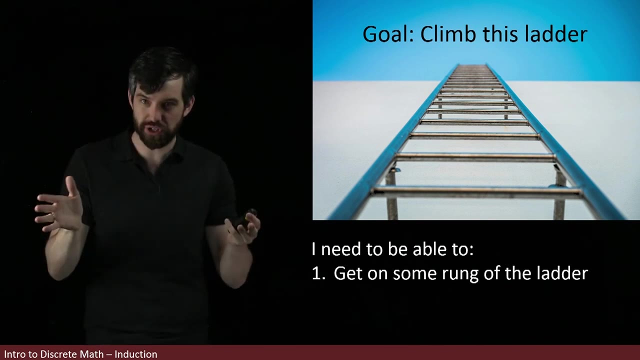 mathematical induction is that of climbing a ladder. So how do I climb a ladder? Well, I claim that there are two steps to be able to climb a ladder. First step: I need to be able to actually get on the ladder. I need to be able to make it to the first rung, or at least some rung. 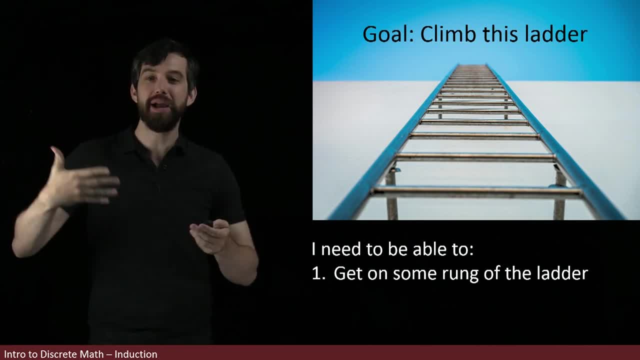 of the ladder. If you've got a fire escape up the side of a building, it might be that the first rung of the ladder is too far above you. You can't get there. So that's my first step. I need to get. 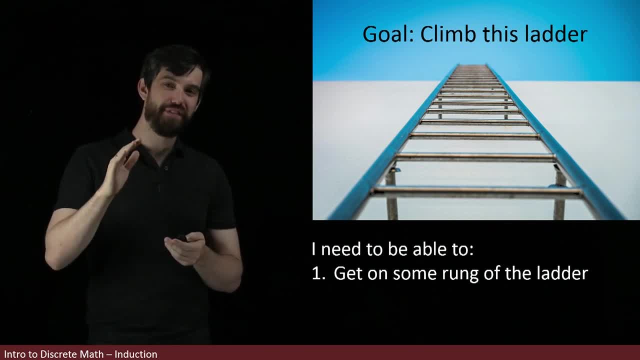 on the ladder. Second step: I need to know that if I'm on some rung of the ladder I can get to the next rung of the ladder. In other words, if I start on that first one and I can go from the 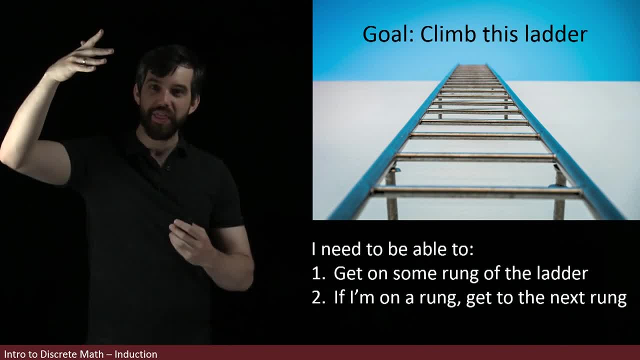 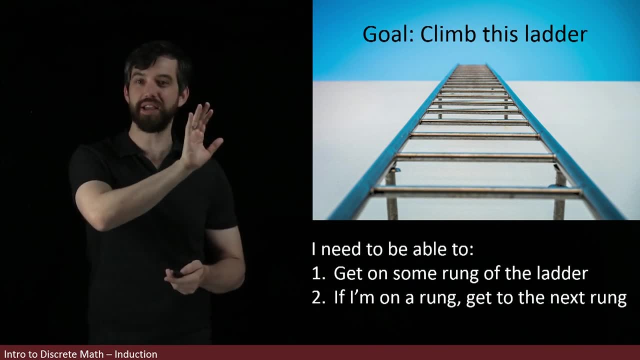 first to the second, then the second to the third, and the third to the fourth and the fourth and so on. that tells me I can climb my ladder, All right, So now let me contrast this with a specific mathematical claim. I want to investigate this big, long, messy thing. It tells. 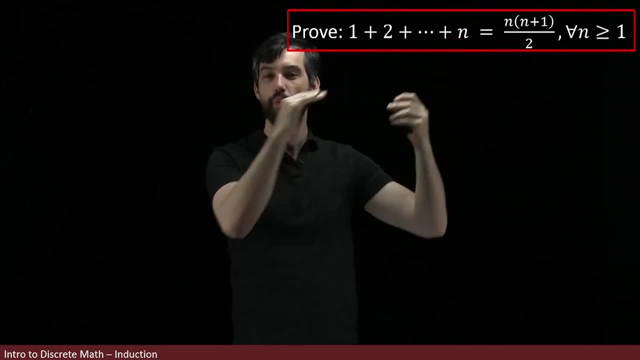 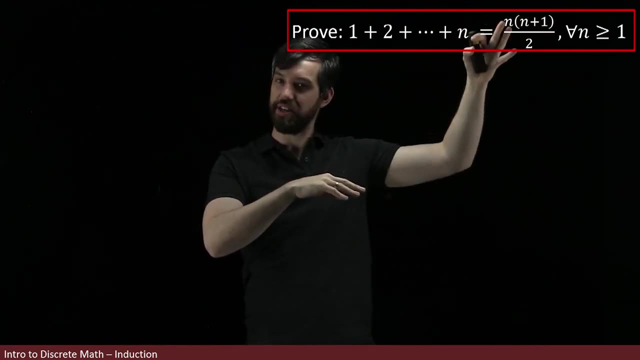 me that the sum of the first n numbers like 1 plus 2 plus 3, up to say 10, that that is going to just be equal to some formula that depends on the final number that you choose here. So for: 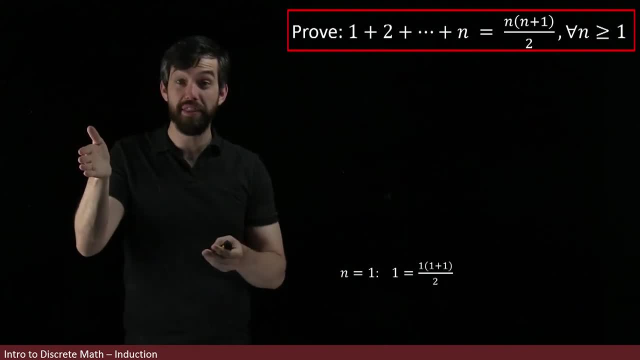 example, in the n equal to 1 case, you're taking the sum of only one thing, the number 1, and it's equal to 1 times 1 plus 1,, which is 2, divided by 2.. This is just a difference. say is equal to 1.. 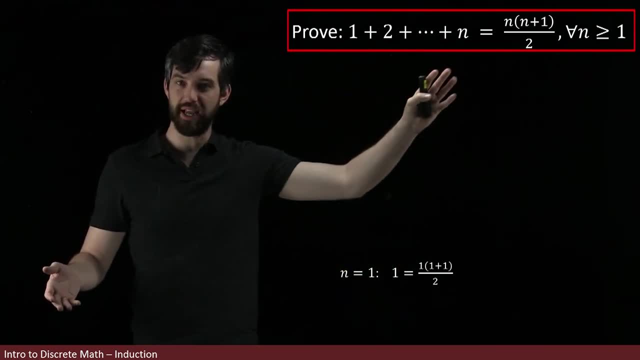 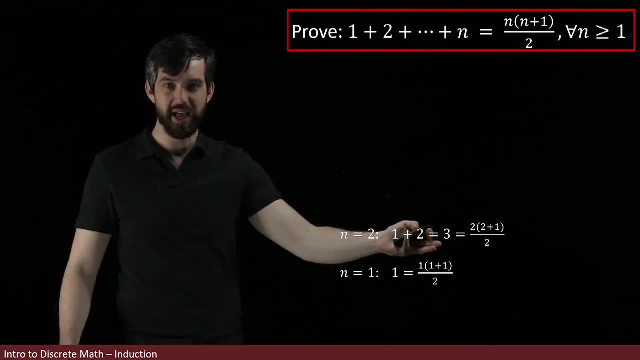 So when n is equal to 1,, this formula is valid, And then when n is equal to 2, it's 1 plus 2.. That's going to be the number 3.. And indeed, this formula that I have over here is 2 times 2 plus 1 is 6,. 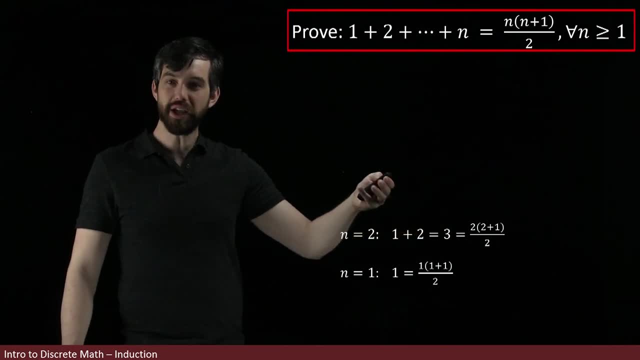 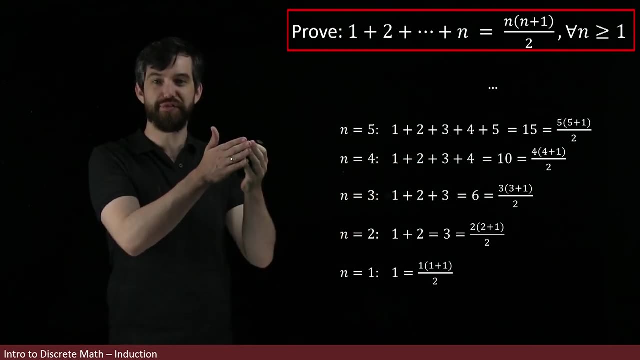 divided by 2 is 3.. So it checks out as well And I can look at what's going to happen in 3 and 4 and 5.. And I can carry on as many times as I want. And the sum, of say, the first five. 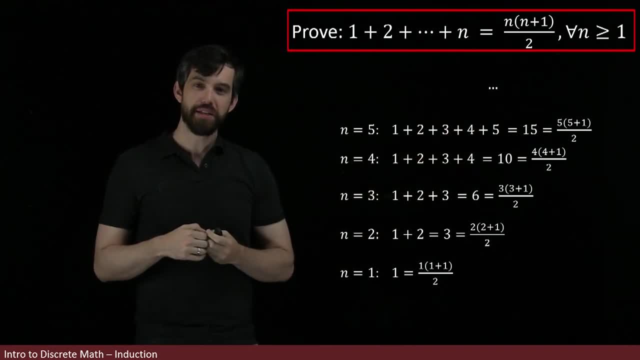 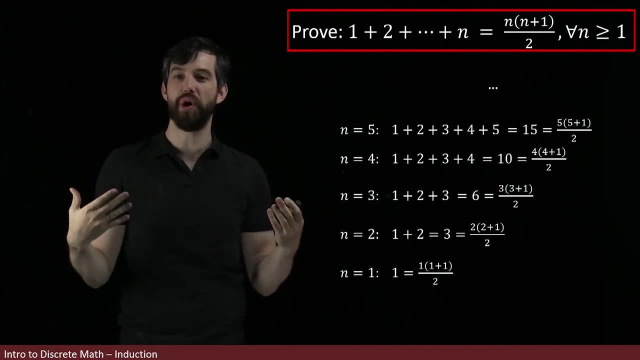 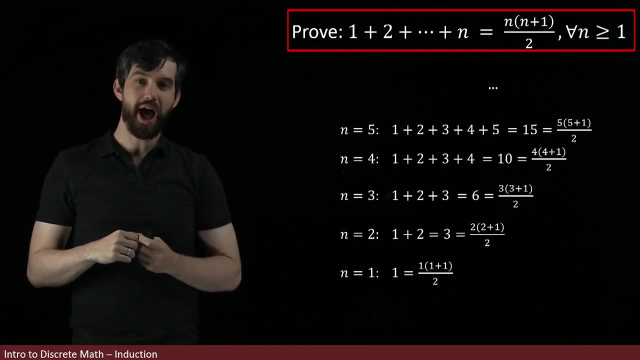 things is going to obey this particular property. So note what I'm proving. I'm proving a sort of infinite collection of claims And I want to do it all at the same time. As in for every positive integer n, starting that's bigger than 1 and going all the way up, I want to have a corresponding. 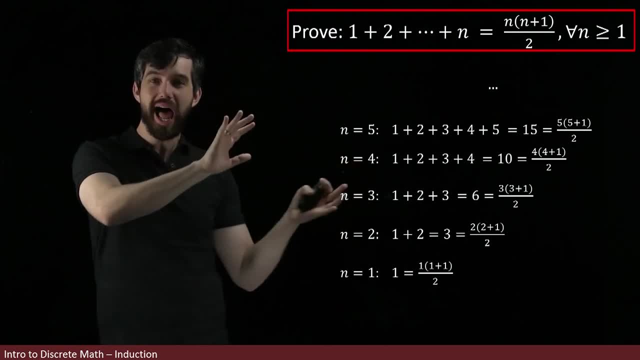 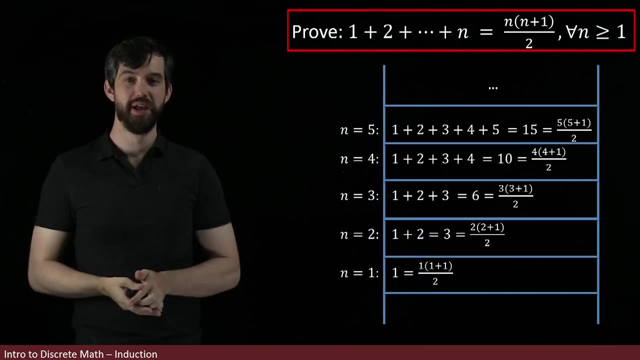 claim. So this sort of style of claim, a claim that is indexed by the positive integers, if you will, it sort of resembles the latter that we're talking about. We're going to say that there's this first step, a second step, a third step, and going on all the way up. Now I have chosen for you a. 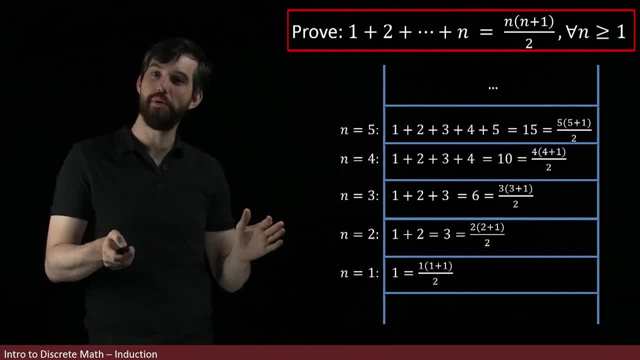 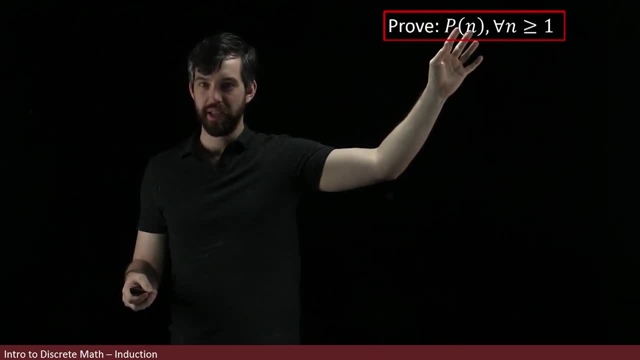 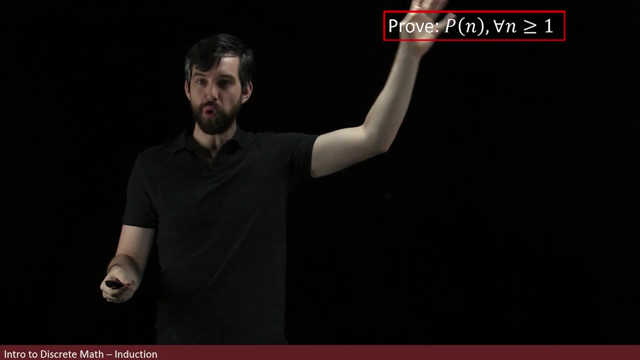 specific example, But we can treat this kind of situation pretty arbitrarily. So, for example, instead let me consider a property, p, that depends on these values, n, where n is going to be positive integer. So in the previous case the property was some equality, that the sum of the first n terms was 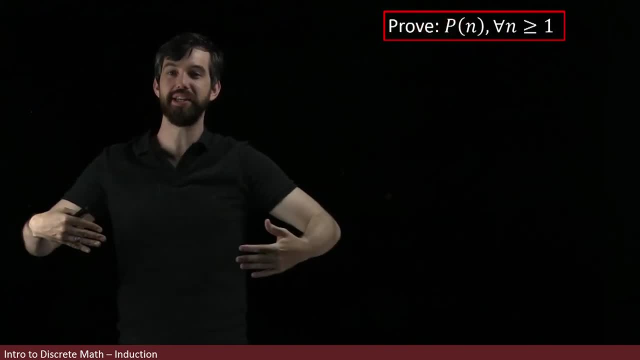 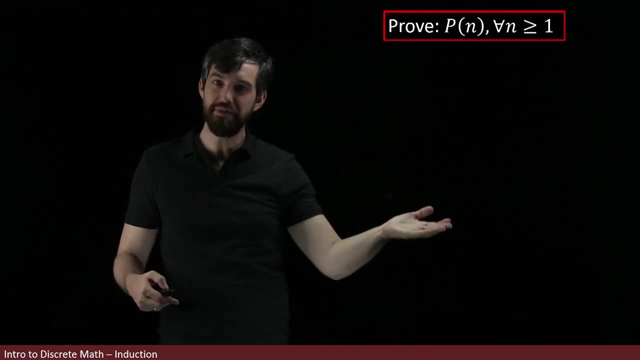 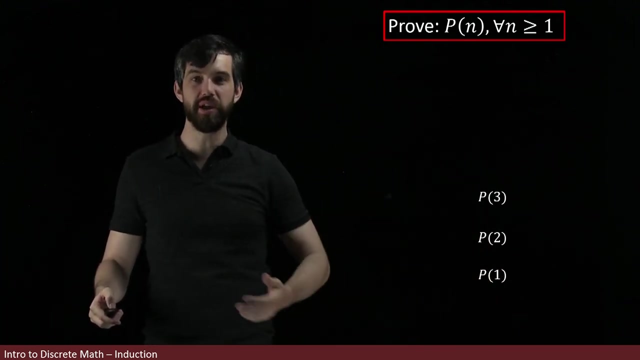 equal to that formula, But this property could just be anything as long as it depends on n or is indexed by n. Then what you get is this infinite family of different claims. You get a p1 claim- That might be some equality or some claim that needs to be true. You get a p2, a p3, a p4,. 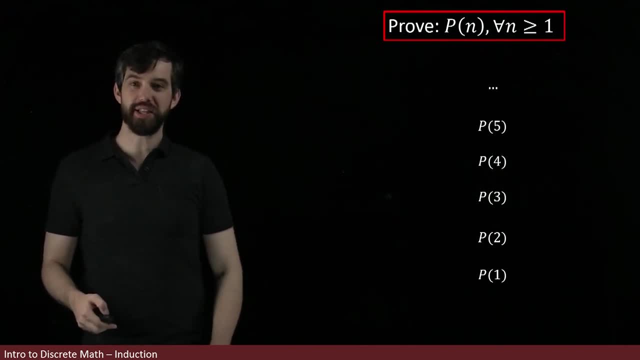 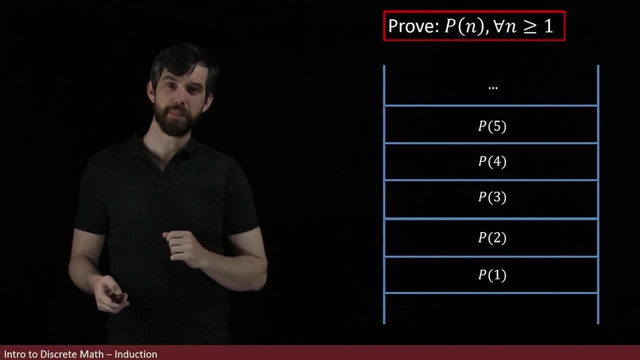 a p5, and so on. So, in other words, the general structure of these claims is again going to be a latter, a first step, a third step, and so on. All right, So let's think: how was I going to climb my ladder? Well, I had to be two different. 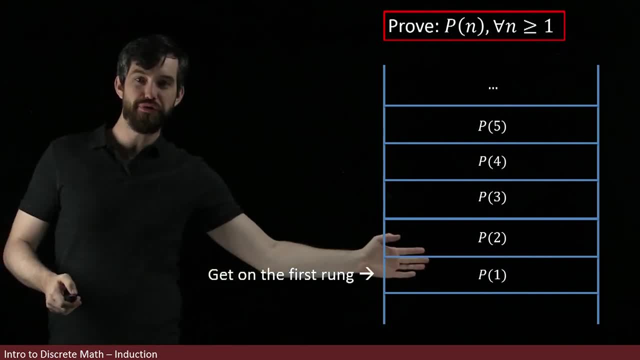 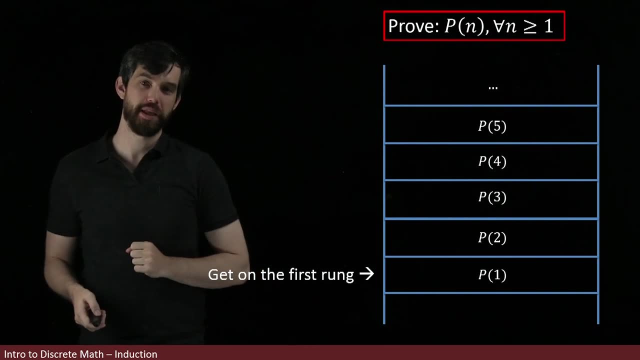 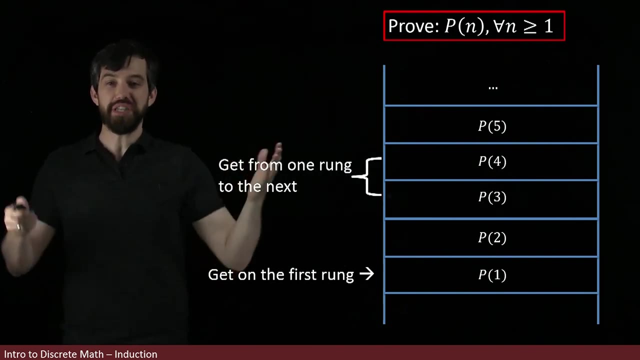 components. The first thing was that you can prove the first of these claims. You can get on that first rung. So I would like to be able to prove that p1 is true. And then I want to know that if I'm on any given rung I can climb to the next one. So I'm going to come here at every step. 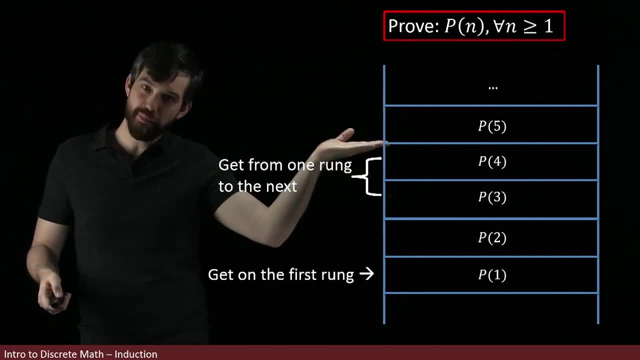 and show that if I'm on, I can get to P3,, I can get to P4.. If I'm on P4, I can get to P5.. If I'm on P5,, I can get to P6, and so on. 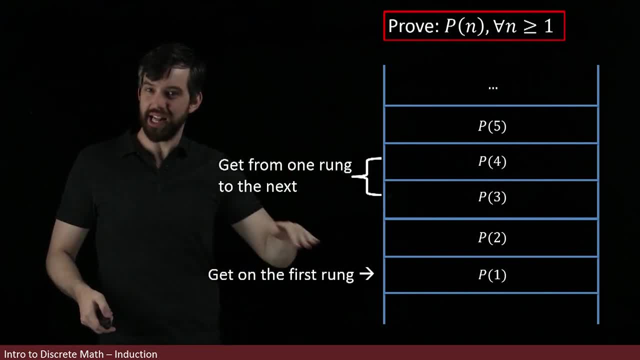 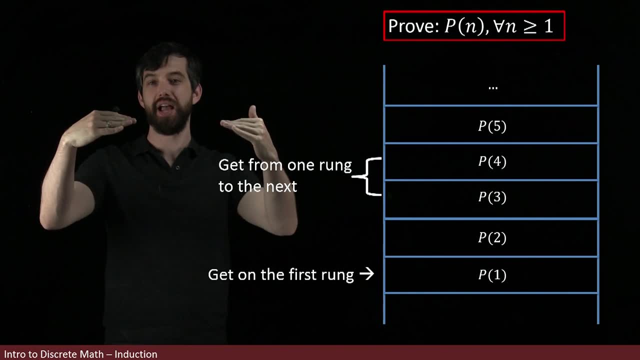 And then if we combine these two things, because I can claim that I can get on the first rung and I can get from any rung to the next one. I can go from one to two, I can go from two to three. 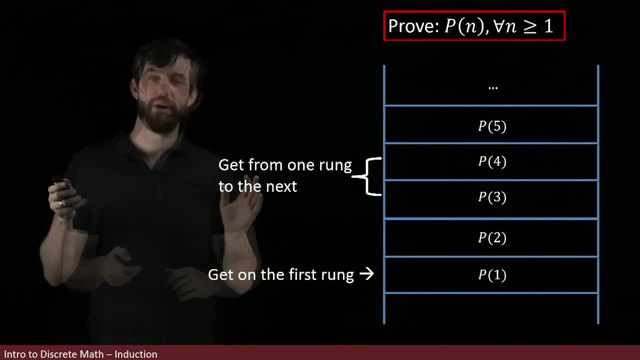 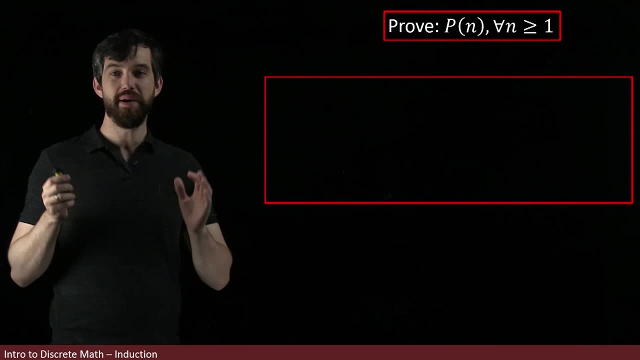 and go to three to four and I can climb my ladder of claims. All right, so let me make this sort of ladder analogy a little bit more precise. I'm gonna claim that my methodology has these two different steps. The first step is: I want to prove. 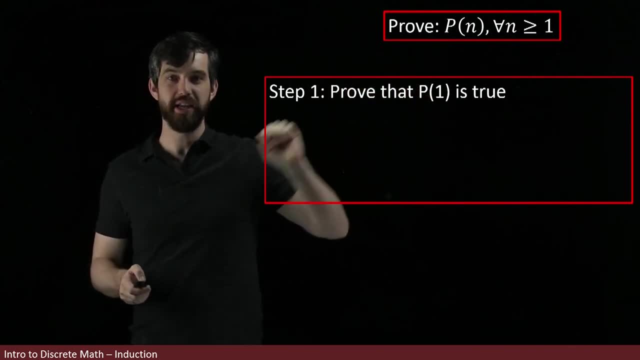 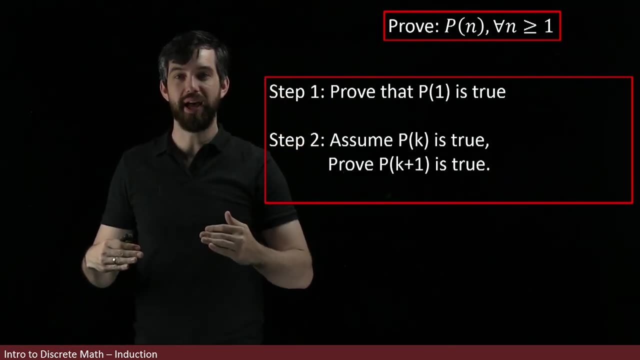 that the first thing is true. I want to prove that P of one is gonna be true And second of all, I want to assume it's true at some level. I use the intermediate value K here as separate from the end of my claim. 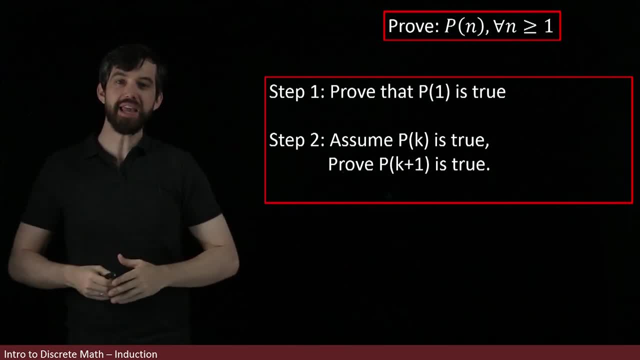 It's just one of the intermediate steps on my ladder And I'm assuming that it's true at the K step and I need to prove that that results in it being true at the K plus one, And I'm assuming that it's true at the K plus one step. 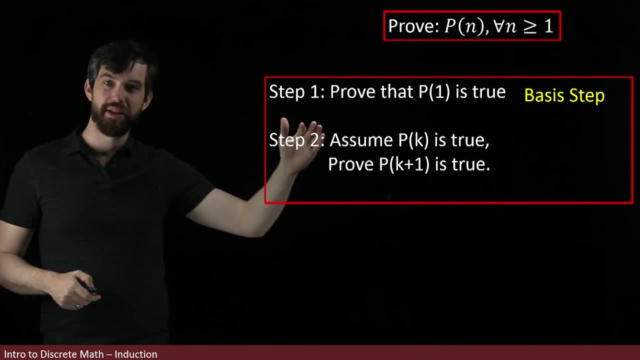 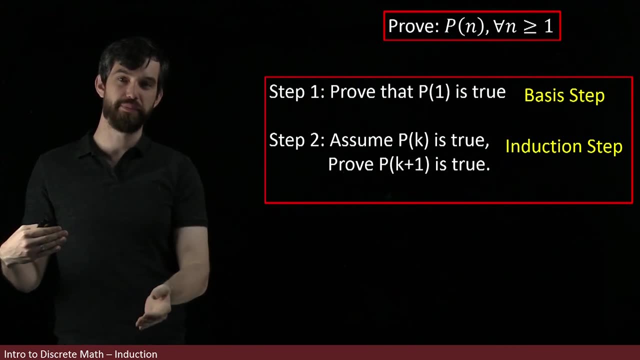 So those are my two different components. The first of them is typically referred to as the basis step, and the second of them is going to be typically referred to as the induction step in mathematical induction. All right now, notice how I started this. 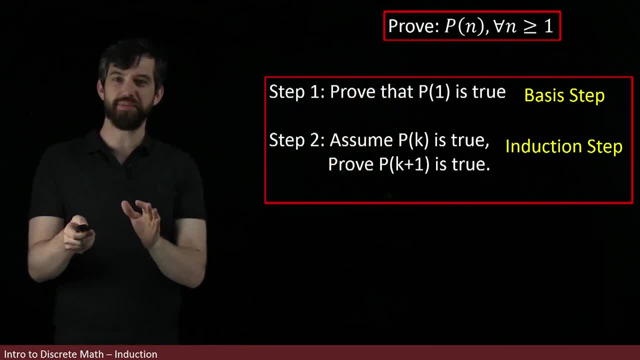 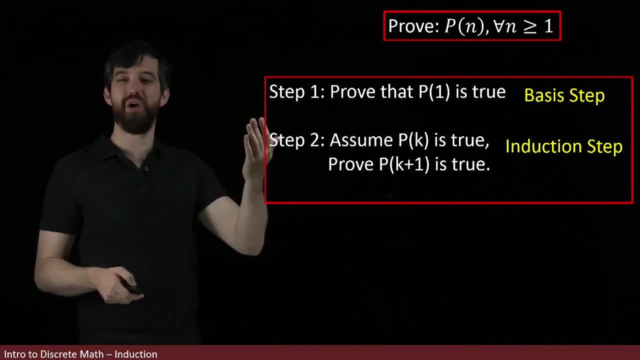 I said, prove that P one is true. That portion of it is a little bit arbitrary. It doesn't necessarily have to be the case that you get on on that first rung. You get on on the 10th rung and carry on climbing. 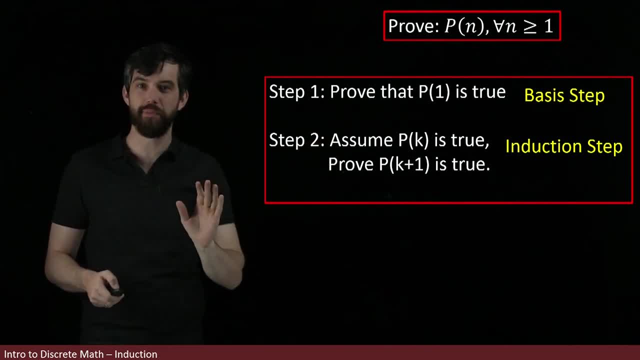 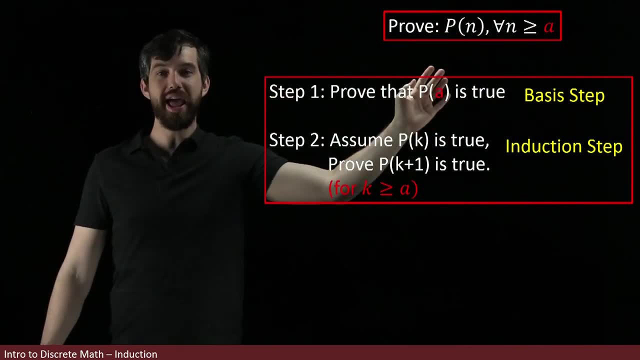 So the general version of this is to replace all the ones here by just some arbitrary integer A. You say, look, I want to prove this for everything bigger than some A. I get on at the eighth step and then I prove this induction step. 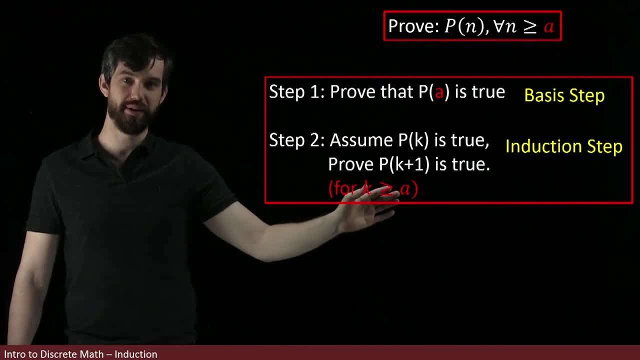 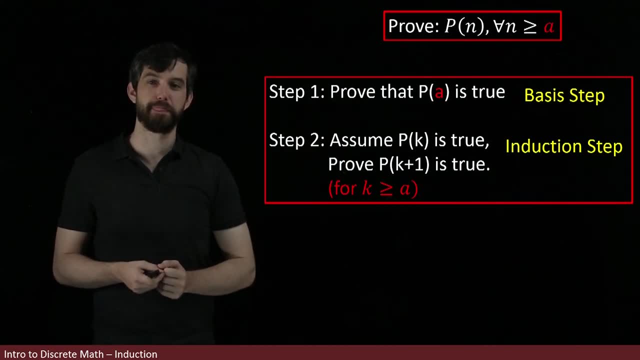 for every value of K that's gonna be bigger than or equal to A. Often, these are structured so that the A is equal to one, but this is the slightly more general setup. All right, So now let's return to the first rung. 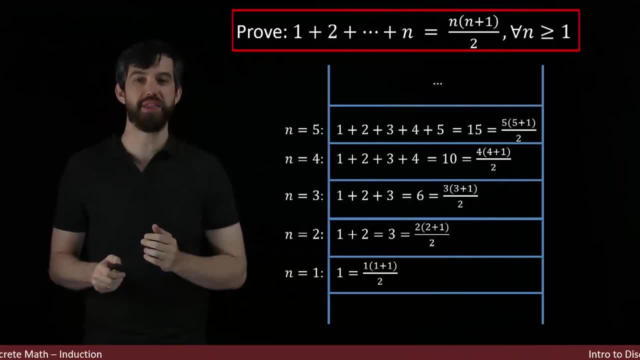 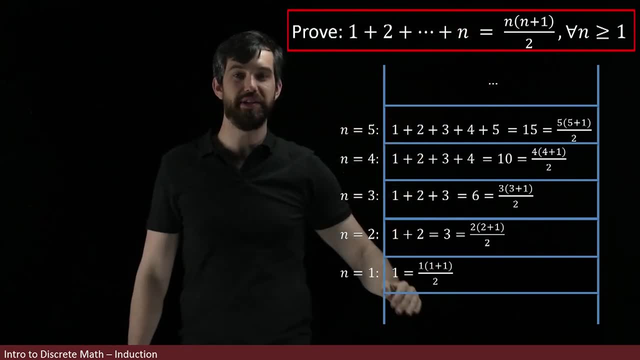 Let's return to what we were proving before. This was going to be the claim that the sum of the first n integers is gonna have this nice formula, and we've divided up into all of these steps, And so what I want to be doing is I want to be proving. 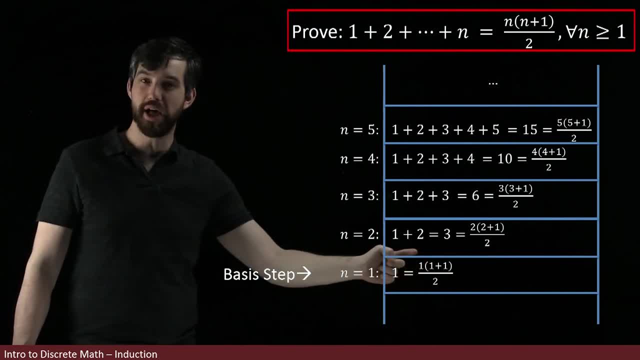 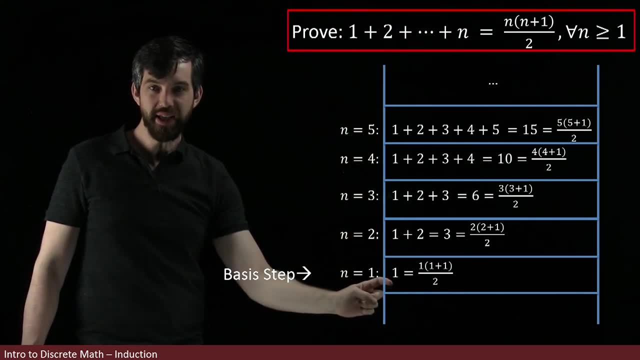 my basis step. that's the first of these, And notice I've already done that. I've proven this claim in the situation where P is equal to one, Why The sum of one thing is equal to the one times one plus one over two, which means 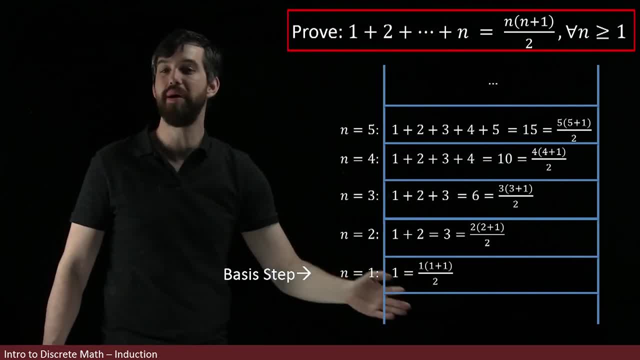 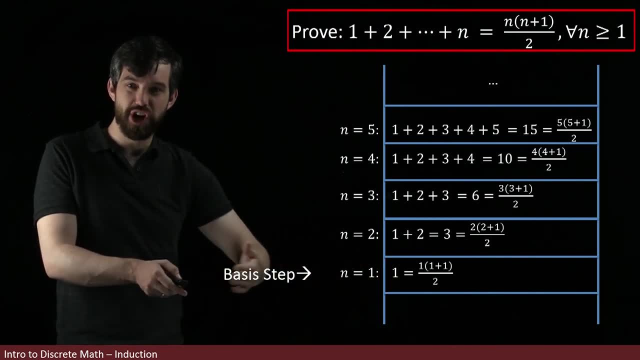 one times n plus one over two in the situation where n is equal to one. So I've proven my basis step already. By the way, it's pretty common that this basis step is a super easy thing. That's generally the case, not always. 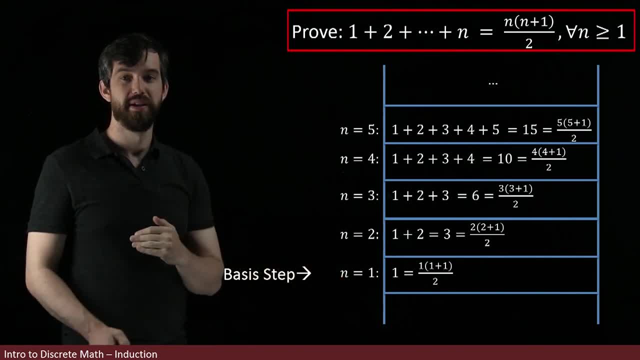 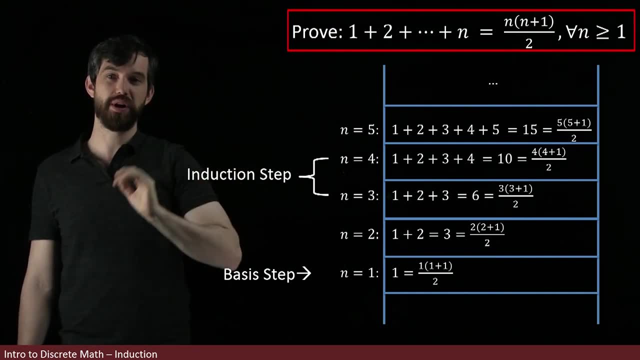 but generally the case, And the induction step's gonna be the hard one. So after the basis step, I have to show my induction step. I have to show how do I get from one level of this ladder to the next. So that's what we're gonna look at now. 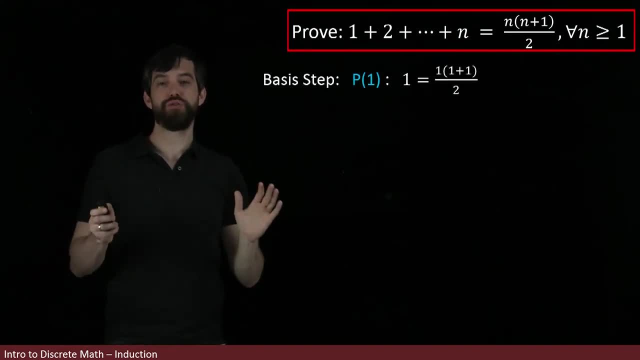 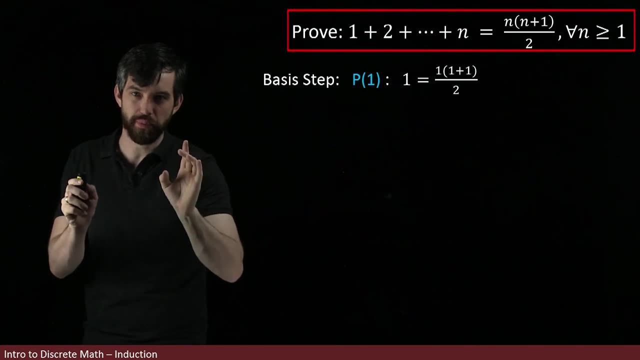 So we've already done the basis step and now what we're trying to do is the induction step. So the way I'm gonna phrase this is: first I want to assume that we have this true for Pk- And what we're gonna assume from our Pk. 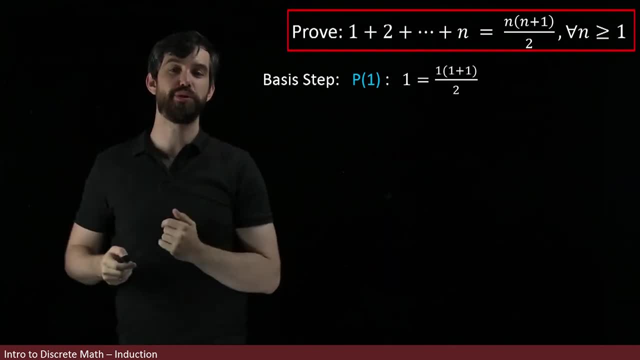 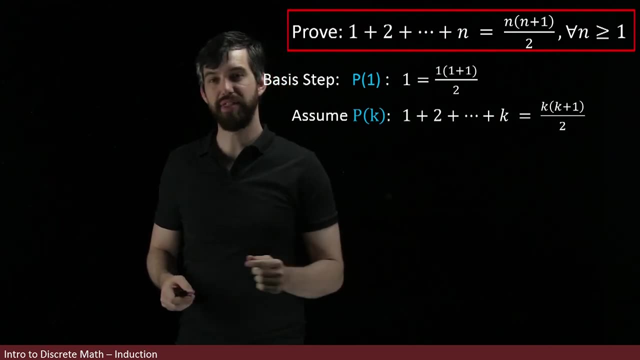 is. we're gonna try to deduce it's true for Pk plus one. So here is my assumption of Pk. I'm assuming that if I choose a specific value of k- if you think about it as running from one up to some value of n- you've chosen some k in the middle. 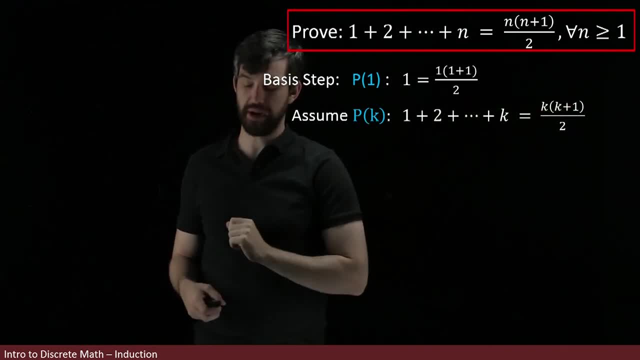 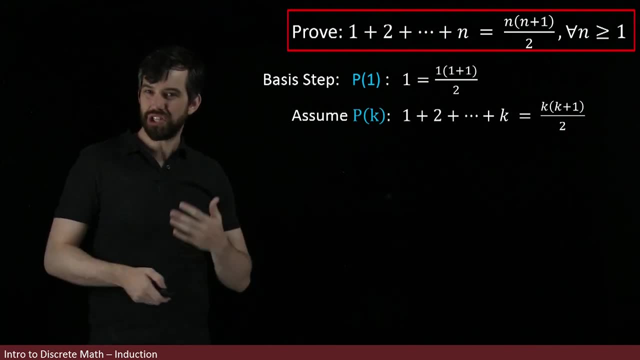 So I've chosen some k and I've said that some of the first k things obeys this formula. Then what I want to do is I want to prove Pk plus one And I'm gonna start my setup like this: I'm gonna begin with the sum of, not the first k terms. 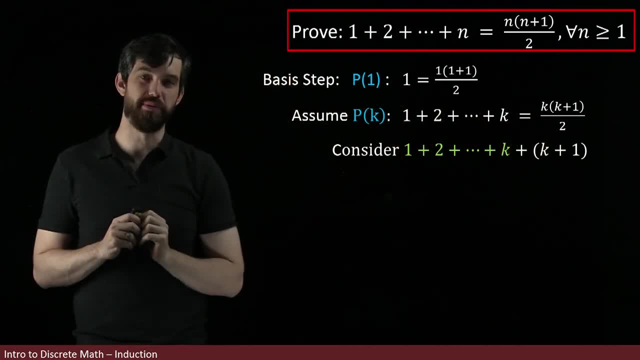 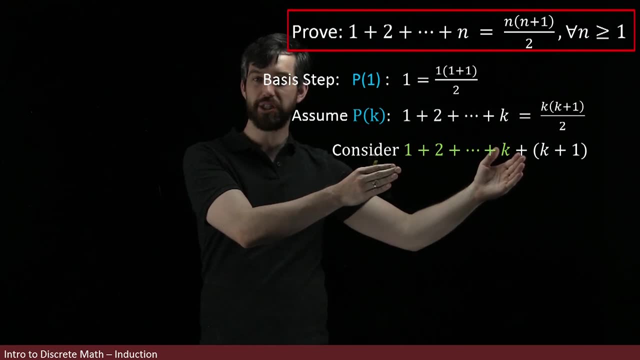 but the first k plus one terms. Now, what can I do here? I know that the green part, the sum from one to k, that is just precisely what we've just seen above, and so I can quote my formula for that. So what this is equal to is: 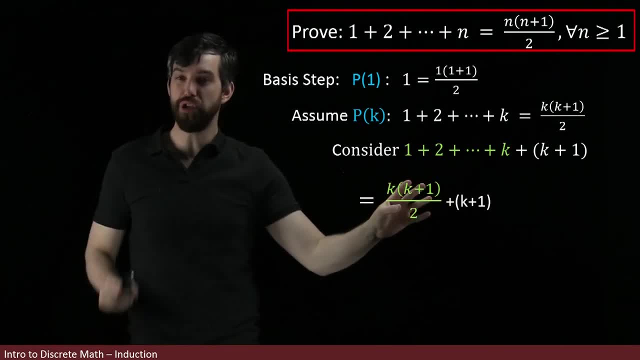 I know that the green part, the sum from one to k, is just precisely what we've just seen above, and so I can quote my formula for that. So what this is equal to is: I'm using my formula, I'm using my assumption. 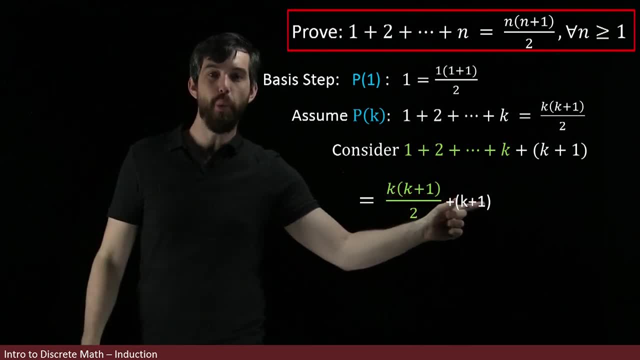 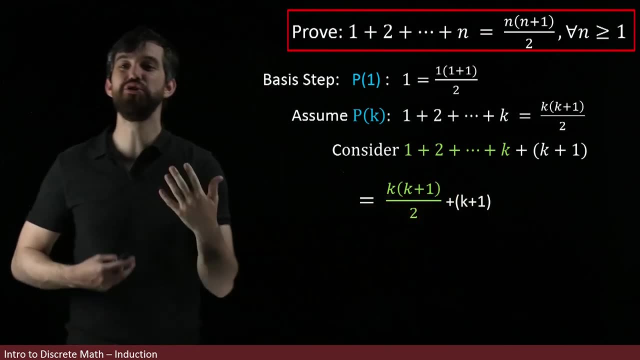 I'm using that induction assumption and then I've got one more k plus one which is sitting on the outside here. okay, Well, now I have this, I can do a little bit of algebra to it. I've got a factor of two on the bottom here. 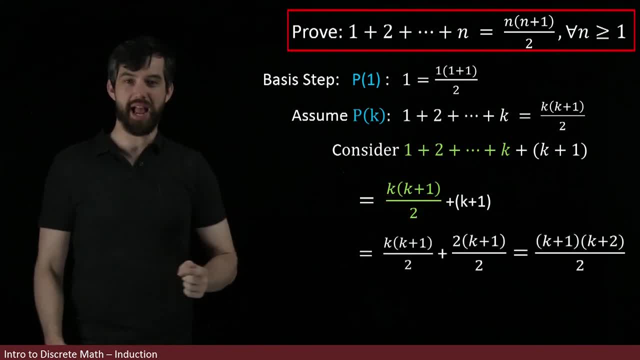 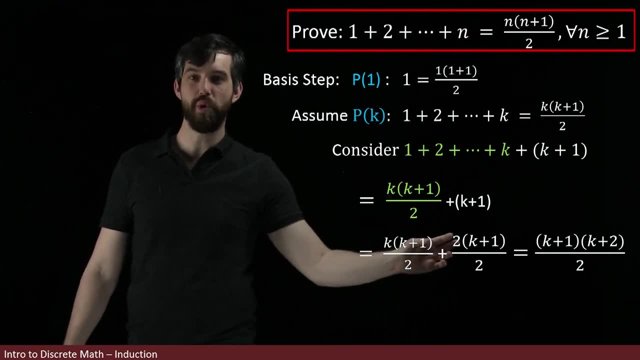 so let's put a factor of two underneath the k plus one as well. I'm gonna do that little trick here, so I multiply by two and I divide by two, and then I'm gonna put these together by saying: look, I got a k plus one and a k plus one. 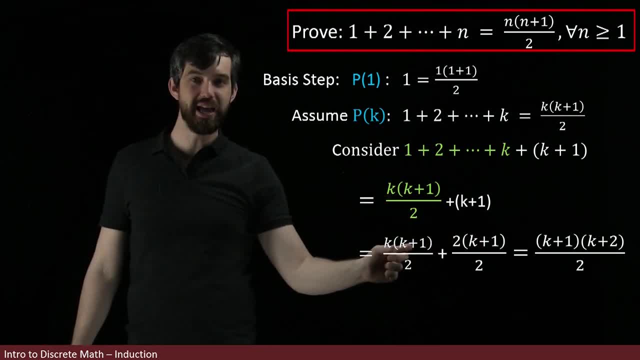 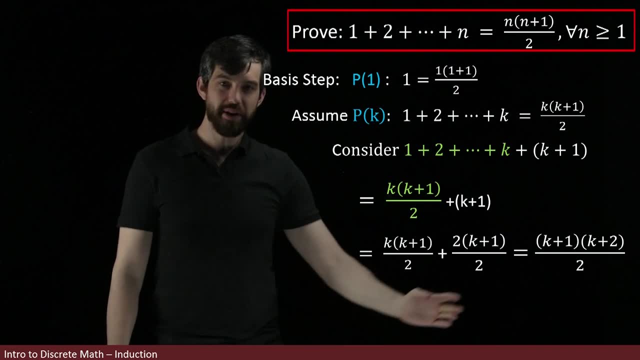 those are gonna come together algebraically. and then I have this k and this two. they're gonna come together and form a k plus two. So I get this little bit of algebra, But this formula that I have here, that's exactly what I want. 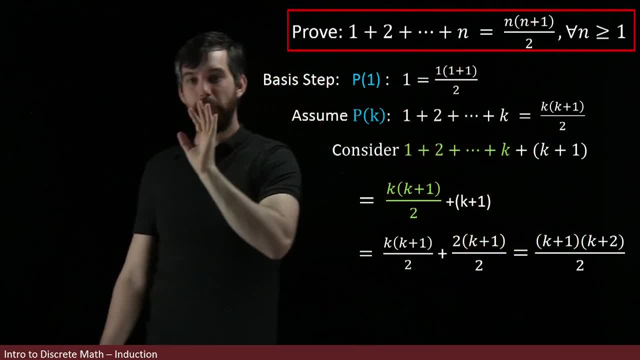 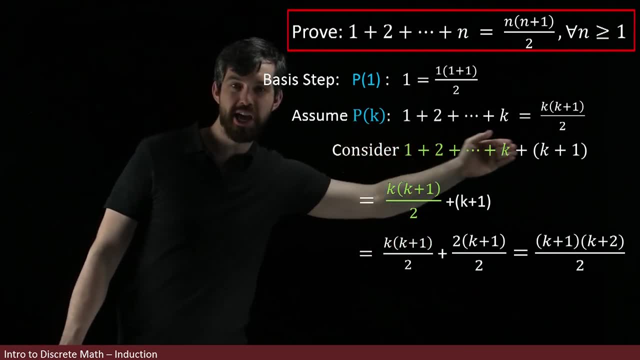 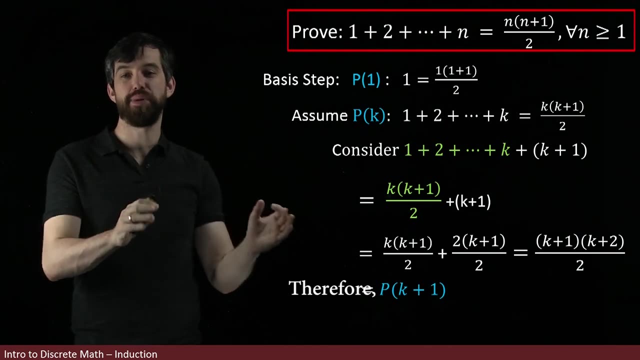 This formula is this one here, but with k plus one plugged in for n. So in other words, what I got is inequality. The sum of the first k plus one terms is that special formula for k plus one. In other words, I have shown p, k plus one. 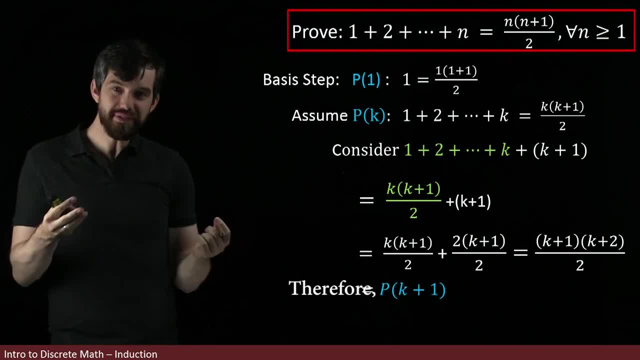 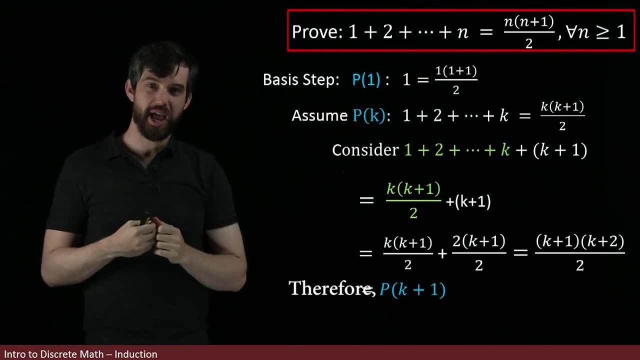 All right. so let's consider the logic of what I've done. I've taken the sum of the first n terms and I want to show that that's gonna be this formula. And I broke that up into these two steps. First, the basis step, where I showed it was true. 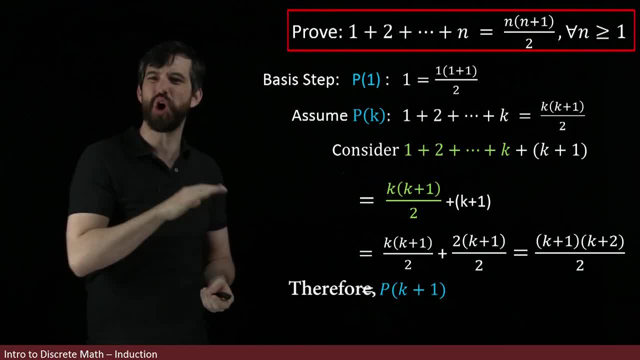 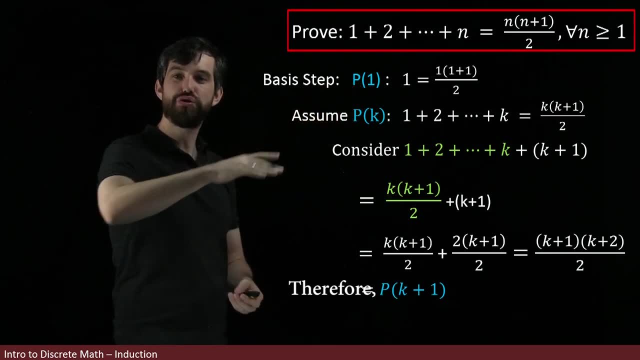 in the first rung of my ladder that for p one it was true and just obviously true. I could just plug in some numbers. Then I assumed this general p k and to try to prove p k plus one I took one side of my p k plus one. 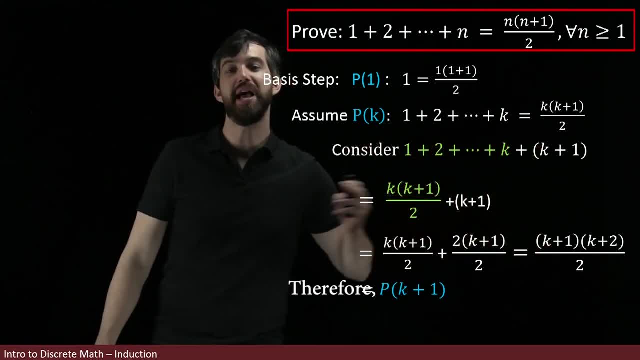 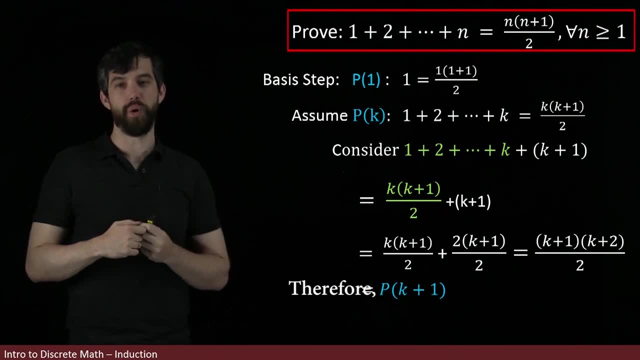 and manipulated using my induction hypothesis to get to the other side of p k plus one, And therefore I claim this claim is true for all values of n greater than one. This turns out, by the way, to not be the only way to prove this claim. 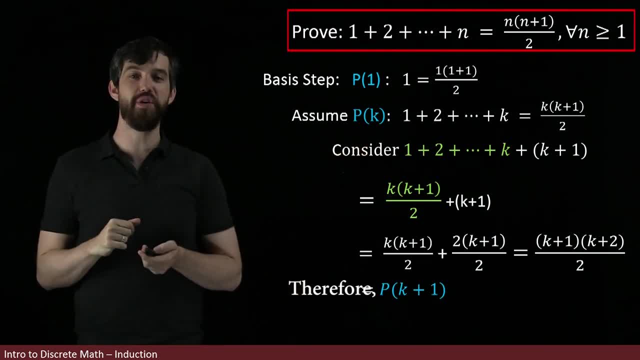 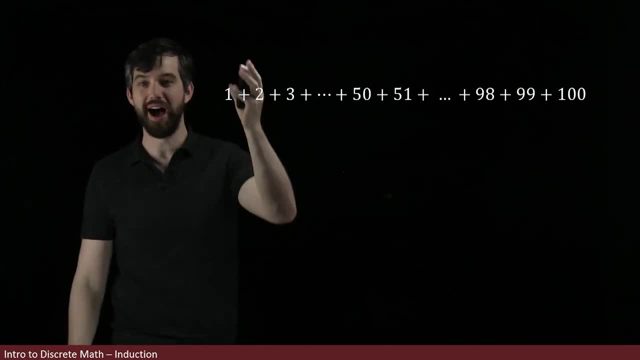 And while it's not an example of induction, I want to show you another way that we can do it, at least in the case for n equal to 100.. So let's suppose that this is true. Let's suppose that I am trying to take the sum. 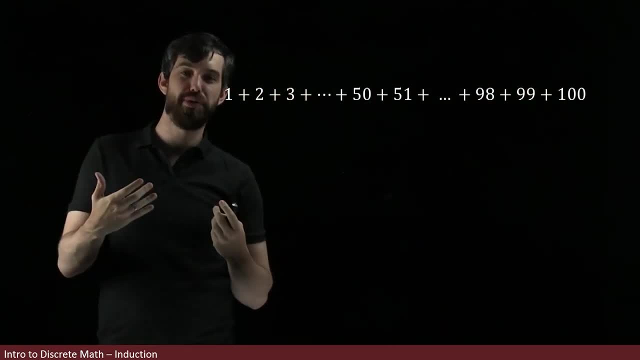 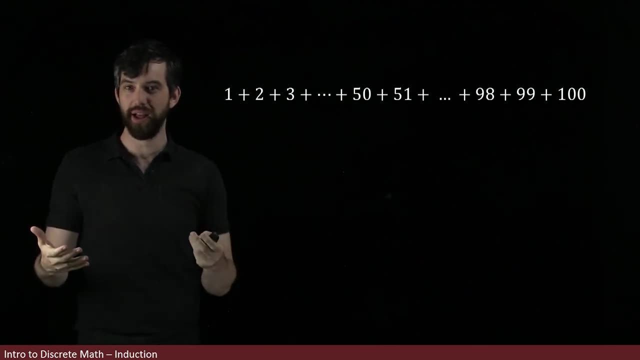 of 100 numbers. By the way, there's an infamous anecdote that goes here, that Gauss, who's one of the most famous mathematicians of all time, that in primary school, when he got in trouble, his teacher told him to sum up the first 100 numbers. 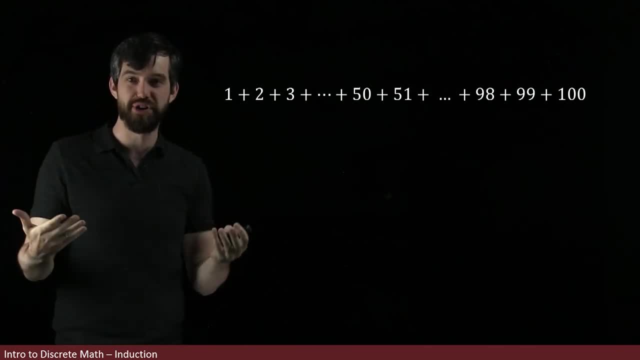 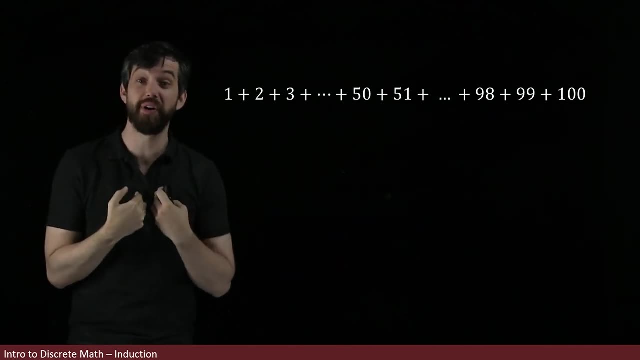 expecting. this is gonna take something a very long time to do. Indeed, if you tried to go one plus two plus three plus, it would take you a lot of time to be able to get to the answer, and we'd all be very likely to make a mistake. 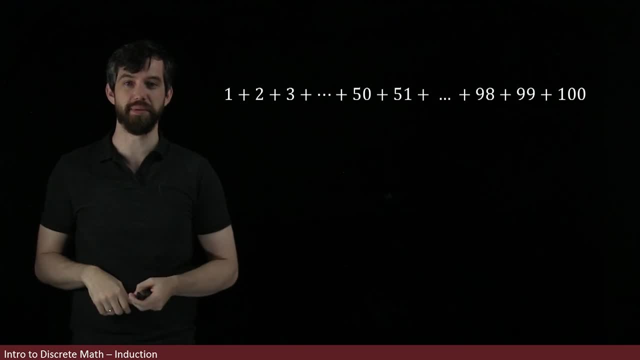 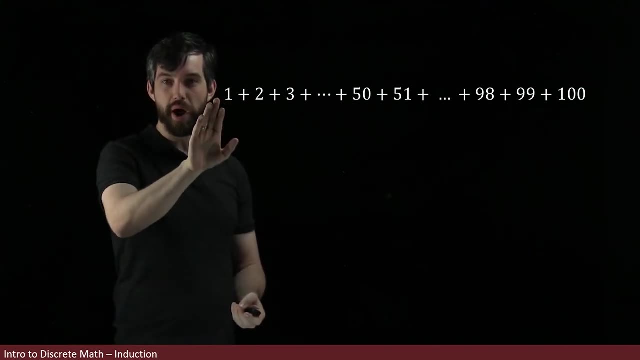 So let me show you a quick way that we can figure out what this is gonna be. Of course, we could just apply the formula that we saw, but I want to show how you could come up with the formula a different way. You see how there's the one here.